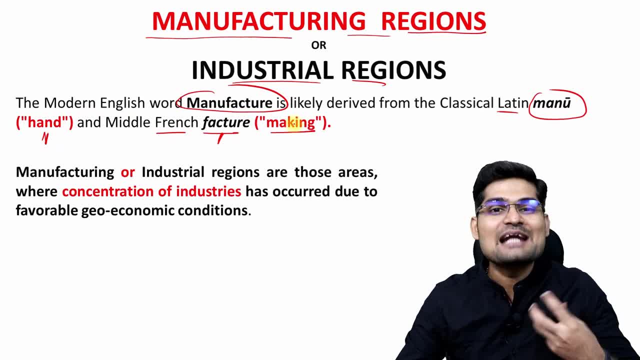 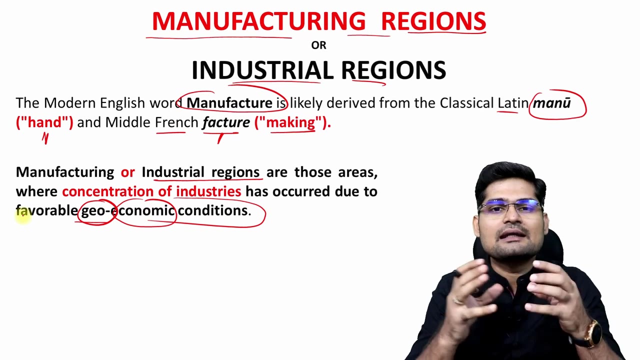 is making. So basically, the word manufacture means what handmade, made by human hands. right, That's the basic idea behind manufacturing. So manufacturing or industrial regions are what? those areas which have a concentration of industries or manufacturing units. that is important And has occurred due to favorable geo-economic conditions. Now two words: geographical and 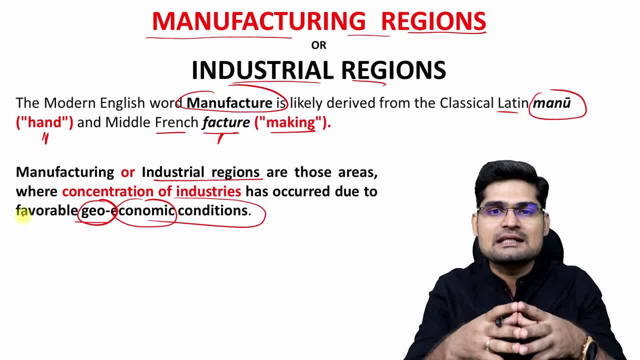 economic. These two conditions, if is their concentrated in a given area and the condition is favorable for the production of or manufacturing of various goods, Then it is supposed to be a manufacturing region. Now the word region, if you observe here, we'll learn in details. 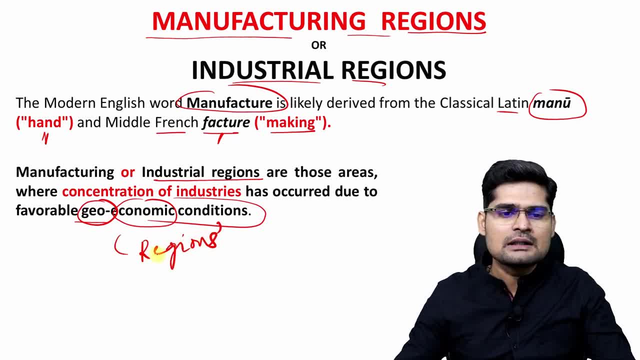 in the lectures on regional planning and development. But for now the word region, wherever you see, The basic idea is it has to be unique in its characteristic and it has to be different from the outside. It means the concentration is different from the outside. So inside and 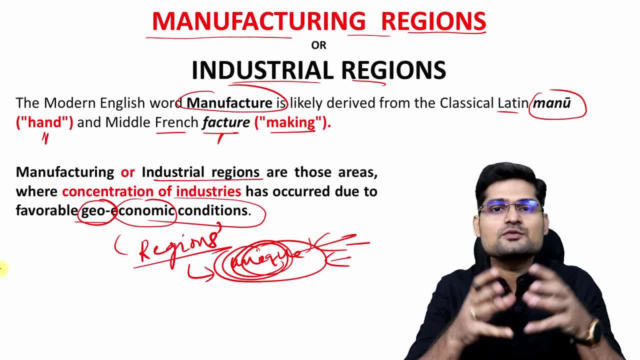 outside perspective, also the uniqueness perspective. that is what makes a region unique. So when we say manufacturing region, it basically means what? it means that that particular concentration of industries or manufacturing unit is different than its adjoining areas or the other areas. Right, That's what makes the manufacturing regions. 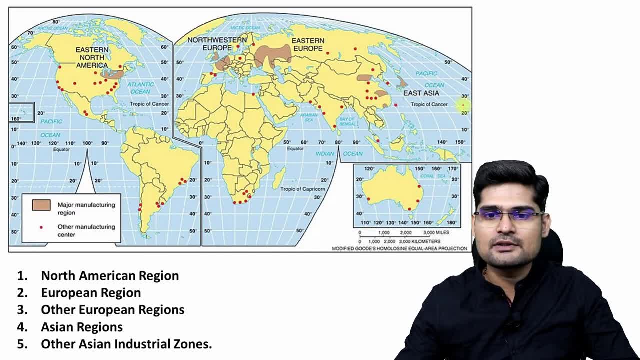 Now let's elaborate and see. So this is the world map here and you can pause the video and you can draw a world map for yourself as well, Or you can take any world map and you can mark these particular regions. So we have five major broad industrial regions across the world. The first one you see here: 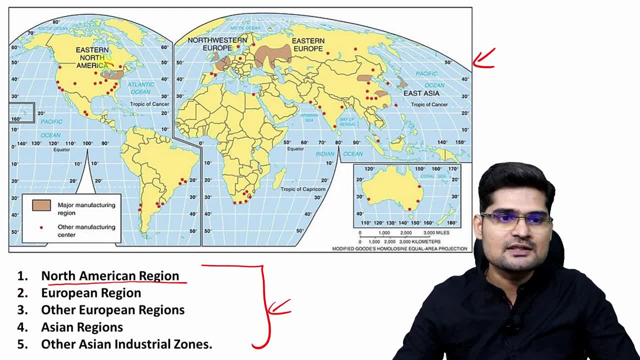 is North American region- Right, So this is where you see the North America and on the west coast and east coast, the Great Lakes area here and also some portions in Canada- Right, So here you will have, in areas where you have the major manufacturing units, major manufacturing regions. then comes 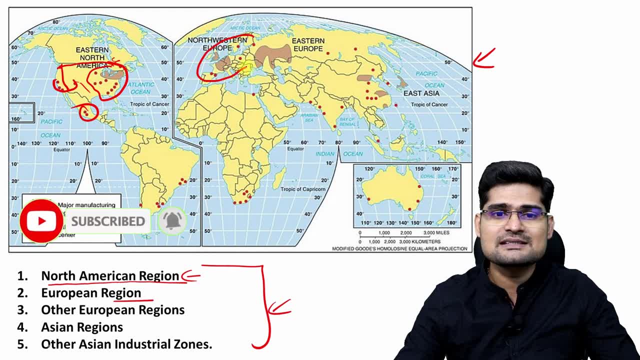 european region in europe, what you see, the western europe. this is the hub where, you see, the industrial revolution began in 18th century, right. so this area again. then other european regions also include the eastern europe right, other portions of europe. then you have asian regions in asia. 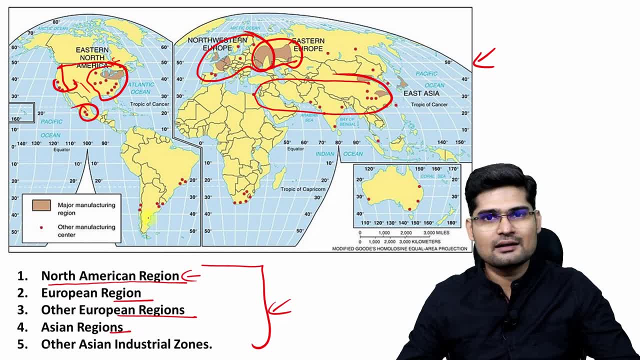 what is there? the entire, this chunk right, including india, as well as china. right and other asian industrial zones also there right in the indo-pacific, singapore, what we say, and some other areas right. so this is what we say, the world picture, and there are certain other. 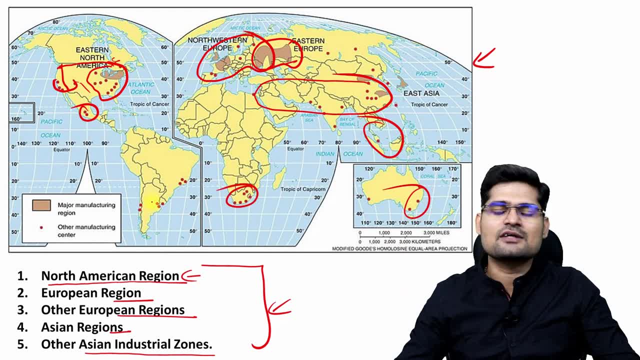 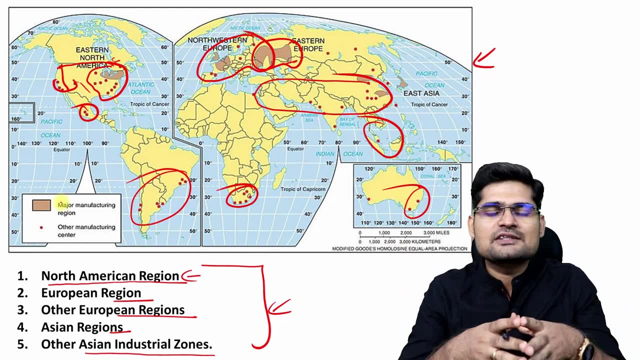 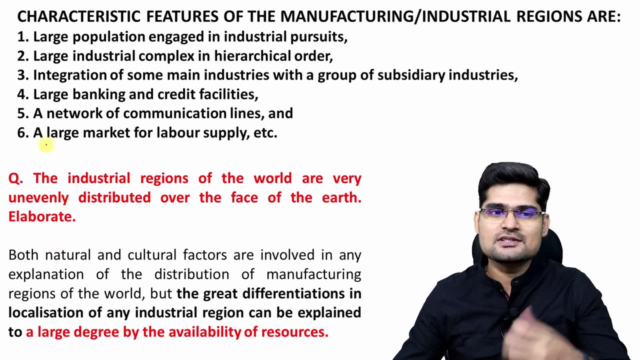 areas. in australia also, you'll have certain industrial hubs, and also in south african region right and also in south america. so these are the major belts in the world where you have these manufacturing or industrial regions. now understand the characteristic feature of these regions, which makes them unique. what are the features? large population. 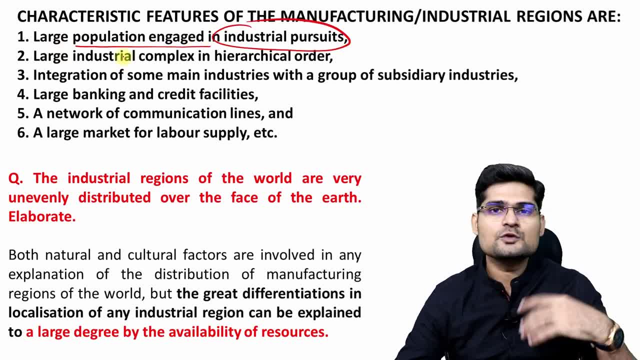 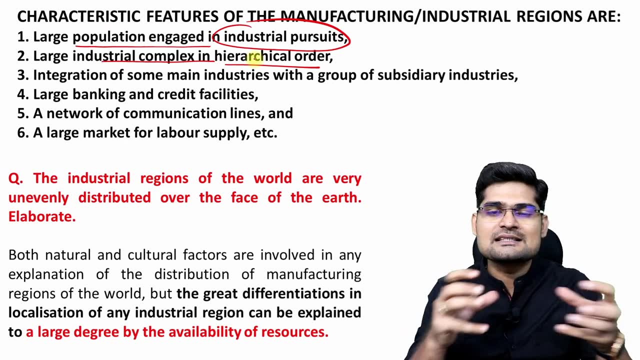 engaged in industrial pursuits. that's the first thing that most of the people- large people, it means, it's a huge population base that is engaged in industrial activity. only right then large industrial complexes in hierarchy right. so remember the higher order settlements, lower order settlements. we talked about these services and goods in central place theory, so more central. 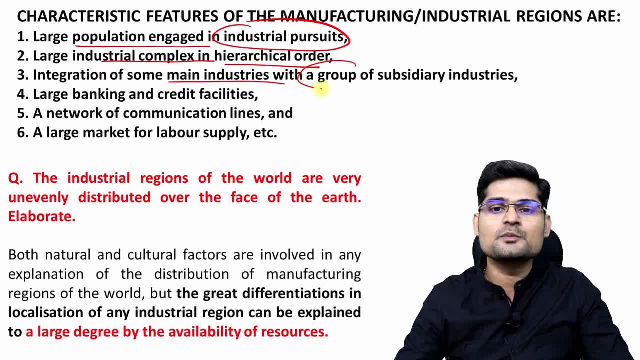 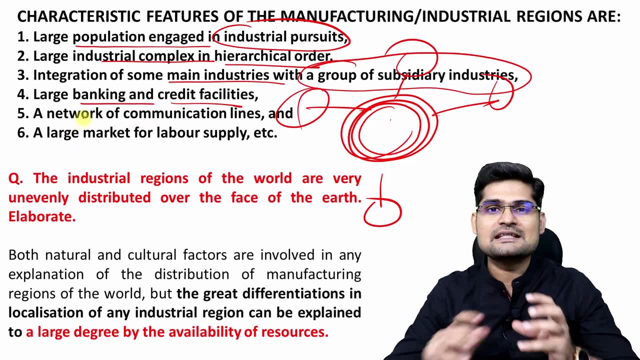 places. right then, integration of some main industries with group of subsidiary industries. right so a main multiplier effect happening on the industrial hub is the large number of industrial hubs that are being built. right so these are the big major industries, so this is kind of an agglomeration. right then large banking and credit. 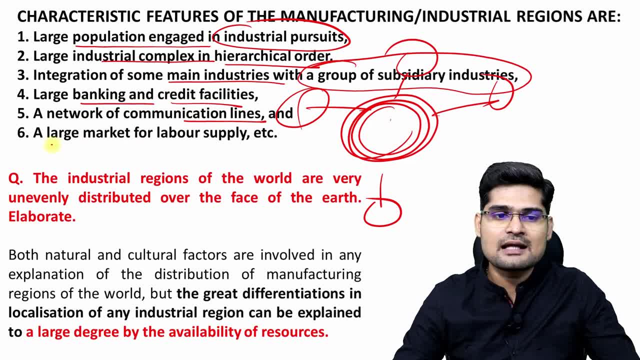 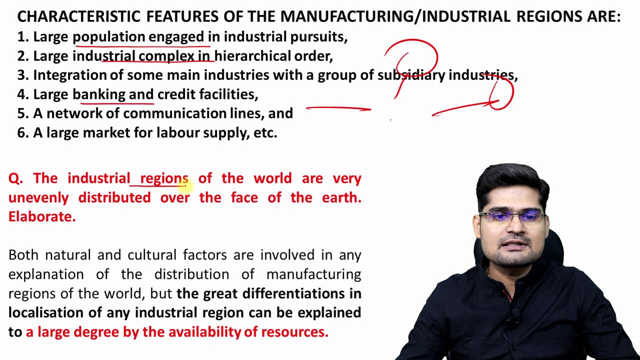 facilities. obviously the environment is given by these facilities for industrial hub to become right and network of communication lines, large market for labor supply. all these things are, must raw material, labor, the factors of production, very important. so now i leave you with a question here. if you observe on your screen this question is what it's saying, that industrial regions of the world. 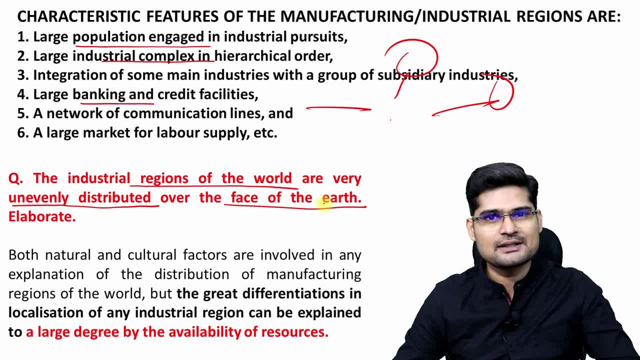 are unevenly distributed over the face of the earth. this is a statement. the word is elaborate with suitable examples, right? so if you know the answer, you can write in the comment box below: right that, why this industrial regions of the world are unevenly distributed? what are the major? 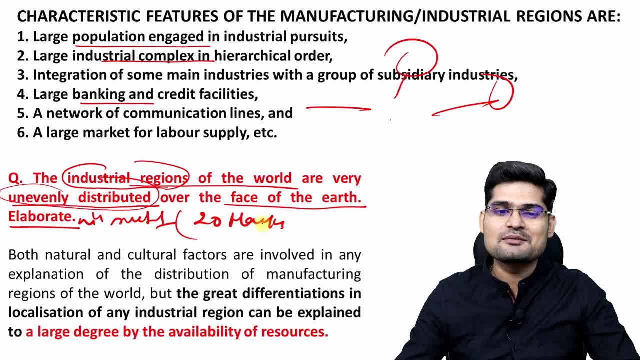 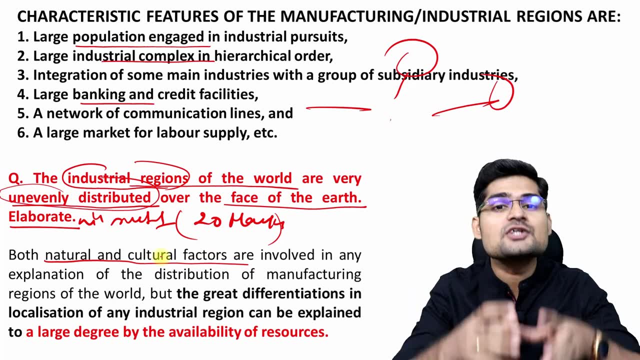 reasons behind it. and if it is a 20 marks question for upsc, think about it. what examples are you going to quote, right? so? both natural and cultural factors, both the factors are important, right? so understand that it's not just availability of land sources or just one factor. it has to be a combination of factors to make it an. 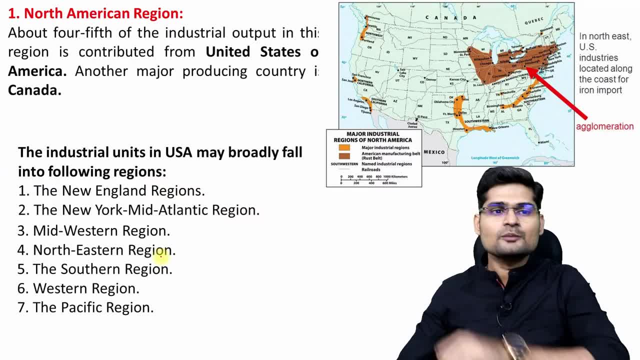 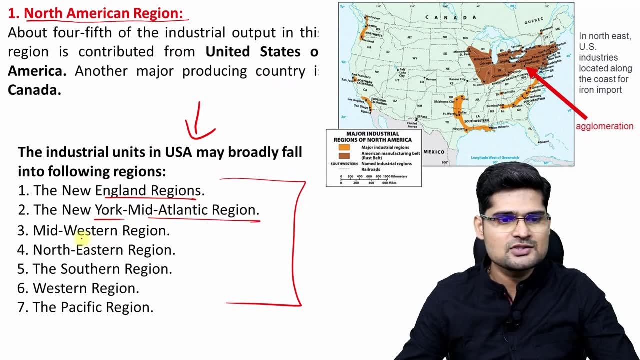 industrial hub or a manufacturing hub, right? so let's elaborate one by one. so first one is in North American region. now look into the North American region. you'll find America and Canada mostly dominating. so in America, what you have in USA, you have New England region, New York, and Mid Atlantic region, Midwestern 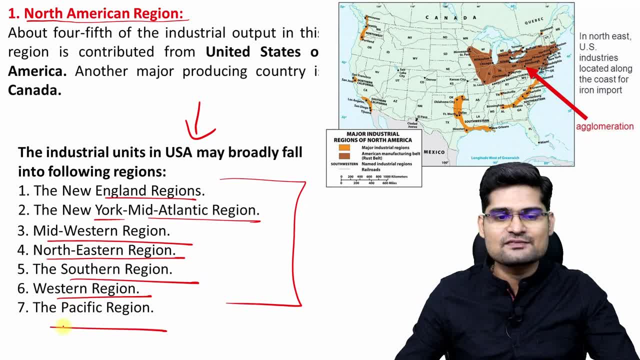 region, Northeastern region, southern region, Western region and Pacific region. seven regions are there and this is marked on map itself. you observe these regions, right, all these seven regions? if you observe, you'll find it here on the map. so this is how you have to practice: with a small map and quickly. 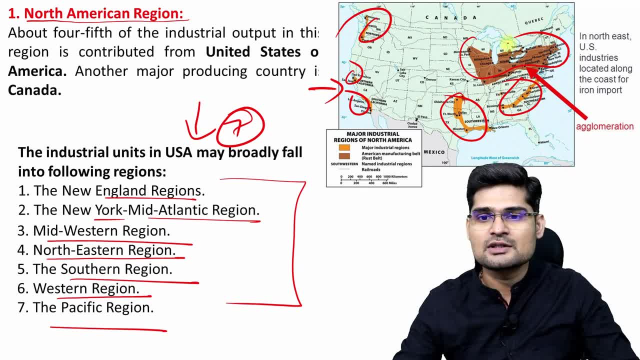 understanding where. which region is there. this is kind of an agglomeration, but concentration is here. this is the bigger concentration that you observe in northeastern portion of the US, right? so this region, the fourth number, is the biggest hub of regions in USA. and now let's look into the Canada, the major. 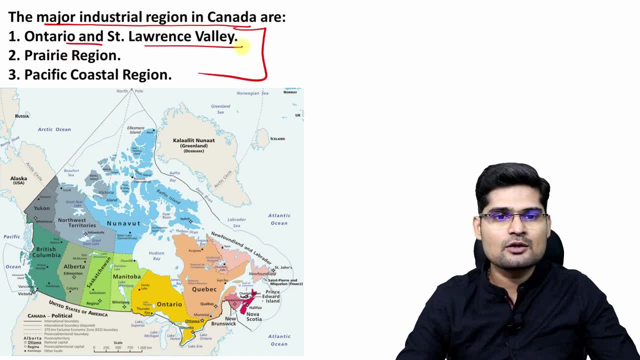 industrial region in Canada are these three regions: Ontario and Saint Lawrence Valley, prairie region and Pacific coastal region. right so, Ontario and Saint Lawrence Valley is the eastern coast, this side. here you have Ontario, this area, then you have prairie region, which is in the central portion, and then 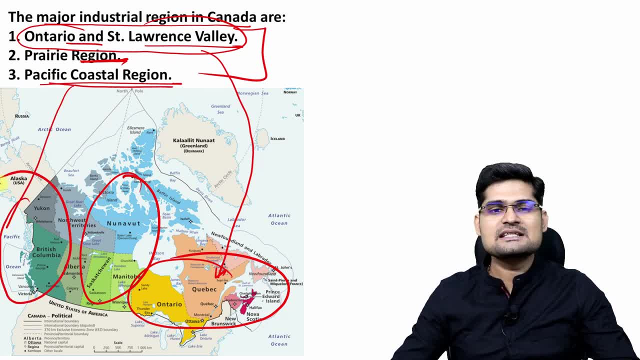 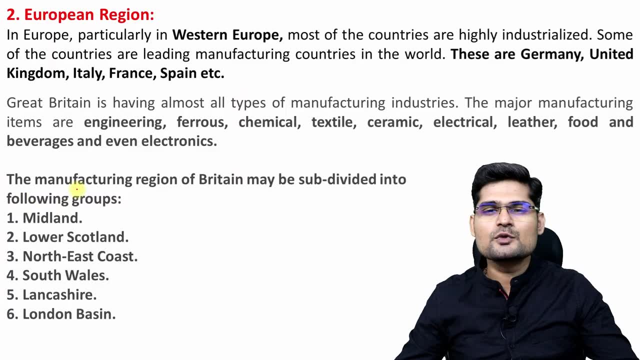 Pacific coastal region is towards the Pacific right. so these are the three major centers or hub of industries in Canada. now comes to the European region. so in Europe mostly the hub is where the Western Europe right. these are highly industrialized, country developed countries like Germany, UK, Italy, France. 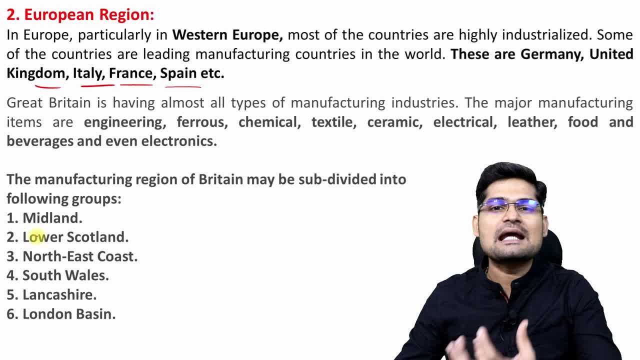 Spain, all of them, and which have great amount of variety of these products like engineering, Ferris, chemical, textiles, ceramic, electrical, leather, food and beverages, even electronics, right, so you observe the diverse city here in Western Europe. so European region is a combination of all these countries where, one by one, if you look in Britain, you have Midland, Lower Scotland, Northeast, 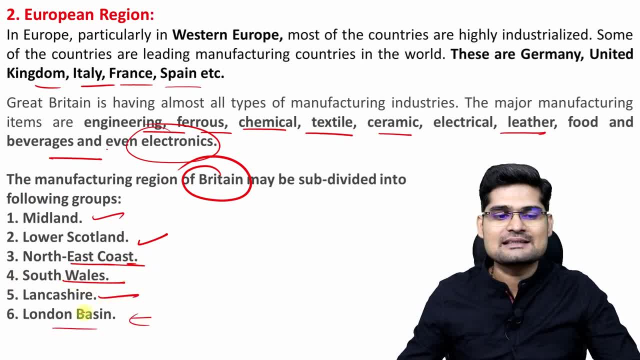 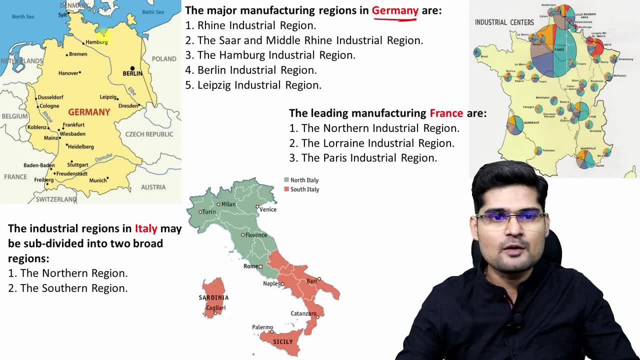 coast, South Africa and New Britain and place in a small population. so this is a south wales, lancashire and london basin. these are the six important hubs in britain itself. then comes to this one, the germany, here right, and if you observe the map of germany here, the rhine. 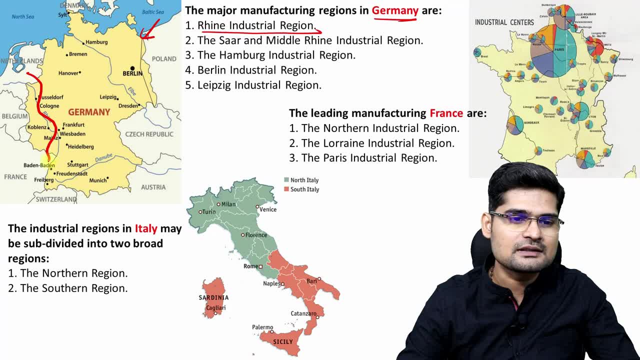 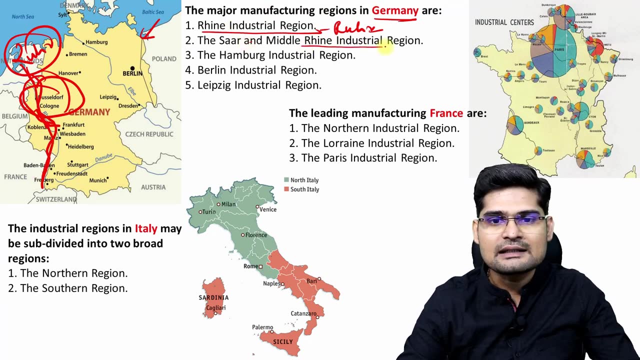 industrial region. now see, this is the rhine river, here this one and this area alongside the rule. this is the rule region, remember, famous for coal, so rule region alongside so rule and rhine region. this you can add here. this region is very famous, then saar and middle rhine industrial region, so 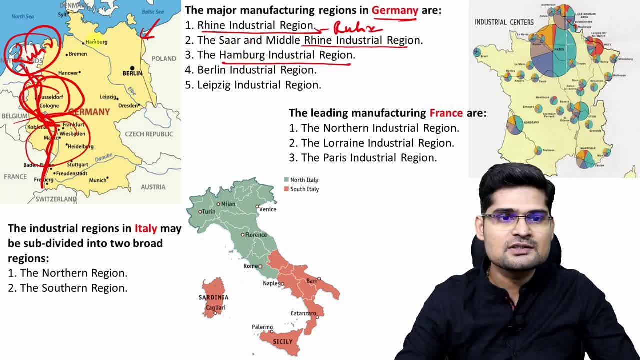 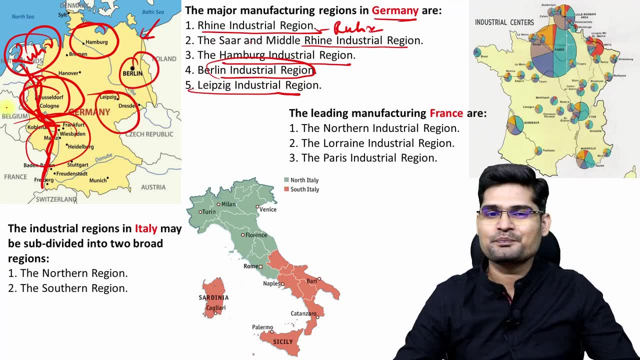 you have middle and saar, then hamburg industrial region, observe in the north here. then berlin industrial region, observe here. and leipzig industrial region- is this one right? so these are the areas in germany that you should work on map as well. now france, if you observe, so northern. 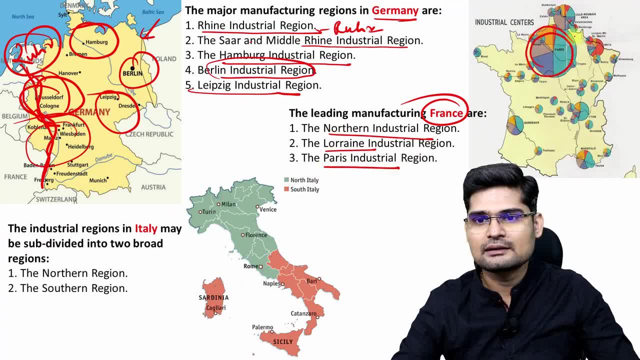 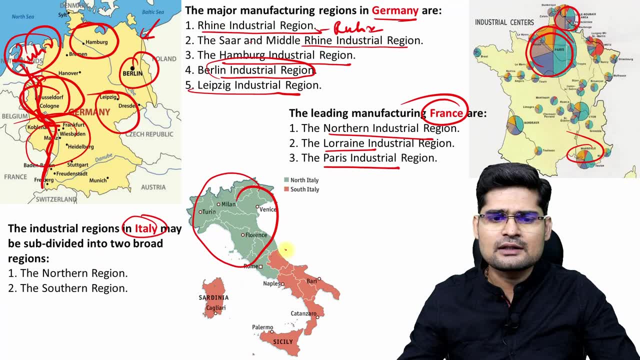 lorraine and ferris. so ferris is the huge one. then you have a little northern and also the others. so right then comes to the Italy. it's very clear-cut south and not divide here, if you observe by colors as well. right, so the northern region is famous for. 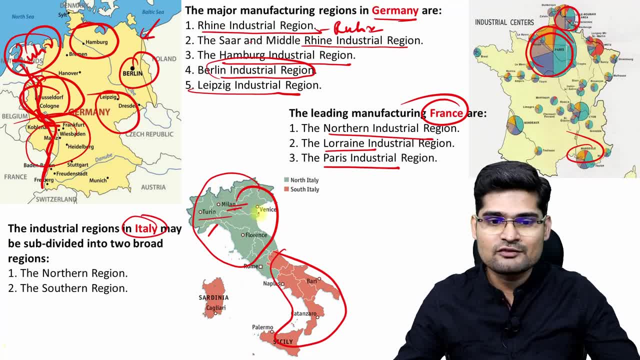 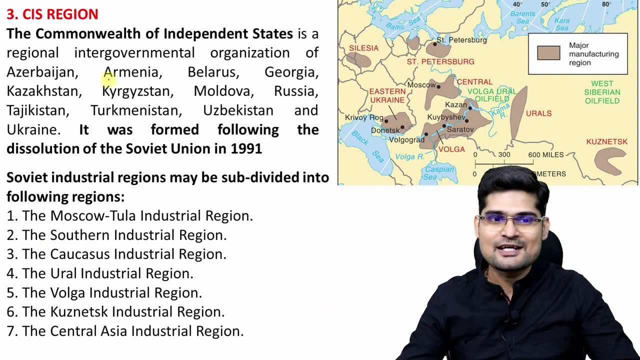 fashion technology, remember fashion. Milan, Turin, Venice, Florence, all these areas, cultural capital, fashion capital, and then in southern, you have other areas which are there. so these are two major blocks. if you observe in Italy right, then comes to this cis region, CIS region. what is this Commonwealth of? 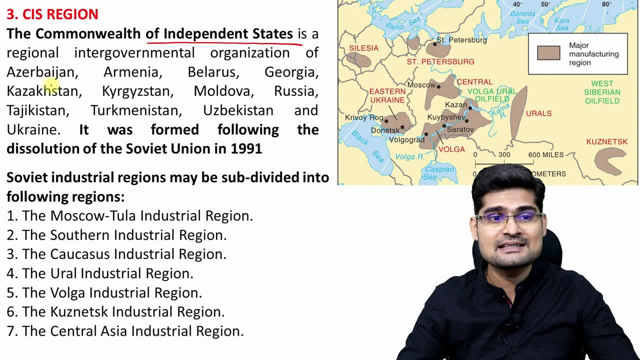 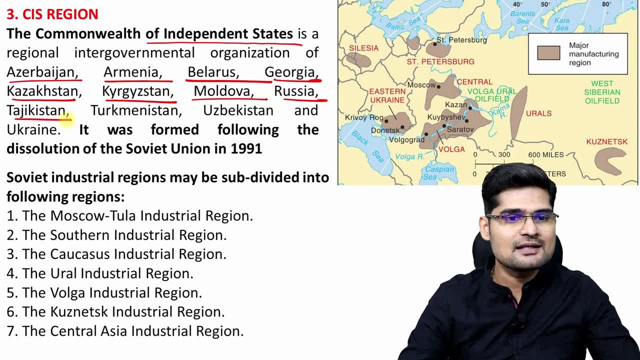 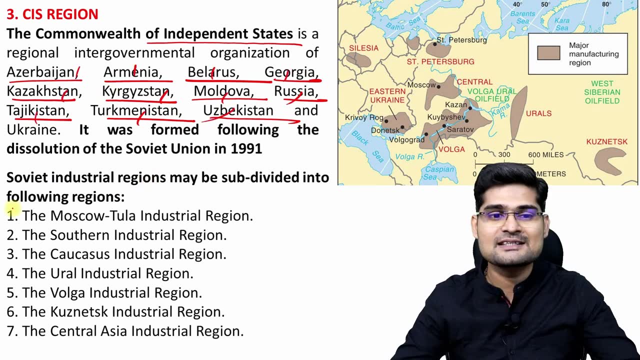 independent states. now, what is this Commonwealth of independent states? Azerbaijan, Armenia, Belarus, Georgia, Kazakhstan, Kyrgyzstan, Moldova, Russia, Tajikistan, Turkmenistan, Uzbekistan, all these countries, if you observe here, coming under this Commonwealth of independent states which was formed by the dissolution of this earlier USSR right, that is, Soviet Union, in 1991. so 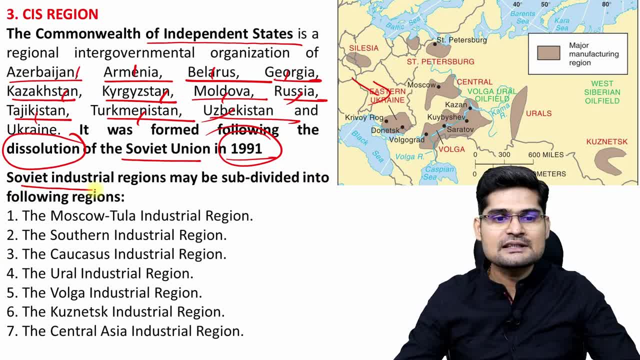 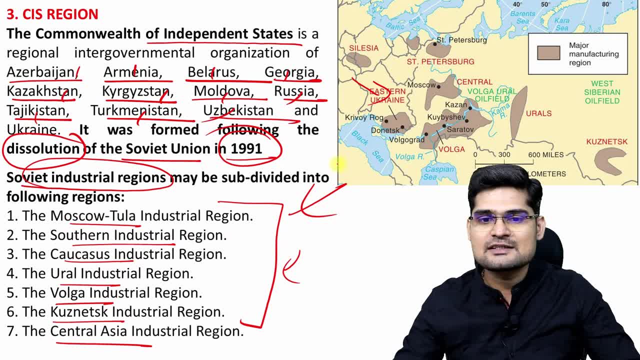 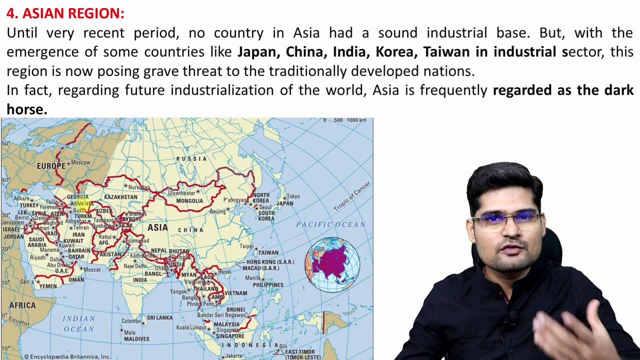 Central Asia, here still region. so this is what you are, the subdivisions and this is the map. if you observe here, so you can look into the map as well and observe these dark spots here, these areas which are the major regions here, which is there right now, come to the Asian one. now, this, I'm sure that being 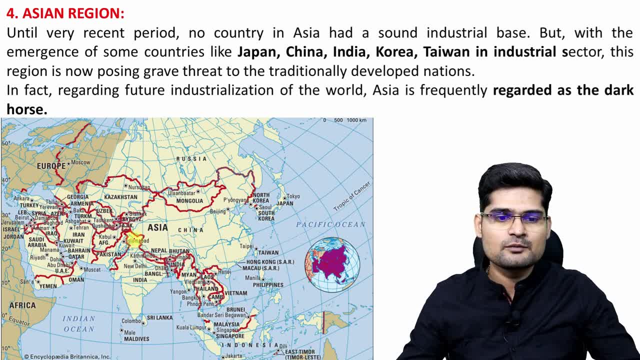 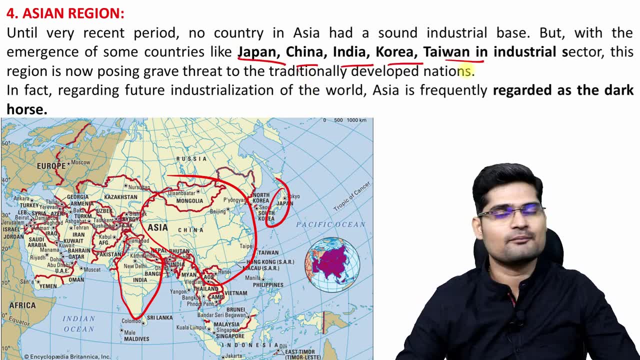 in India and you are more familiar with this region as well, because here the divided between china and india. so do you observe? japan is one industrial hub. china, india, korea, taiwan, right, the major ones. then one more thing that is important: that this region, the asia, is. 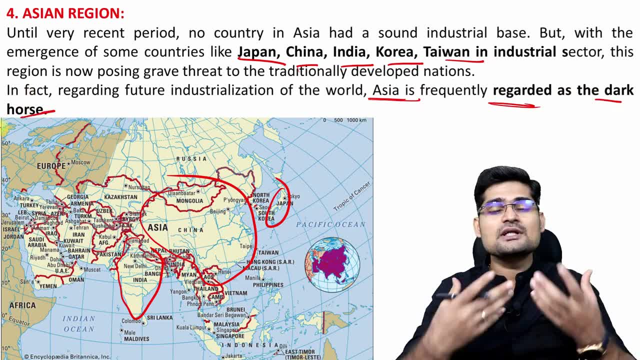 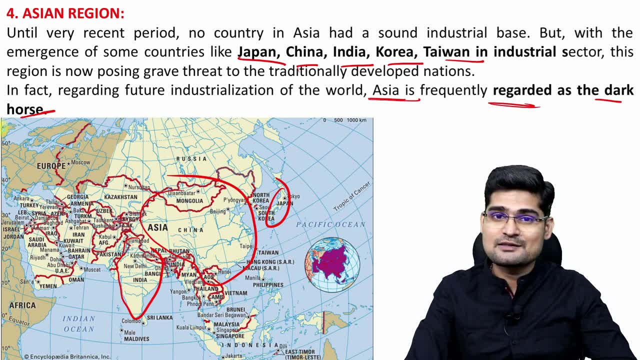 frequently regarded as the dark horse, because the future industrialization and also the market is here. huge amount of population, right. so that's why it's also called the dark horse region that you can remember now on the basis of concentration of industries and their output: chinese industrial. 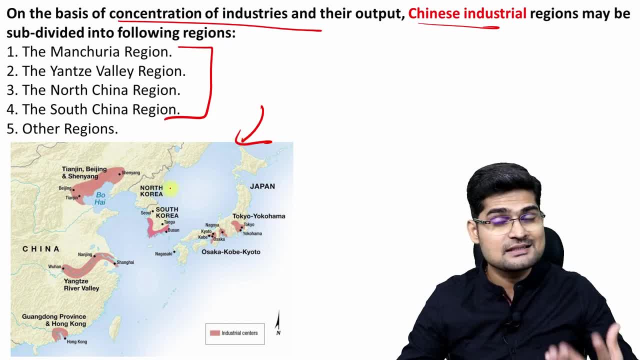 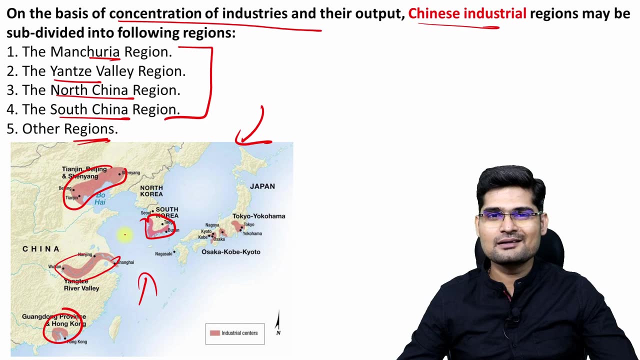 regions can be further subdivided. if you want to look here how china is leading charts in terms of manufacturing: manchuria, yangtze, north china, south china and several other regions, observe it here. these are the major regions in china where you have their industrial hub. right, that's where china 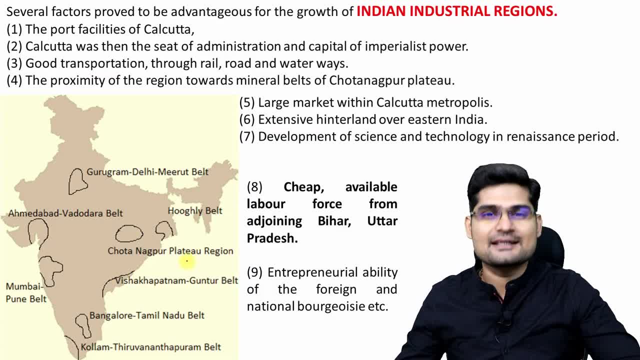 is producing. all the goods now come to the indian industrial region, which we have also looked in the previous lectures in the secondary sector of economy. here what you have is these seven to nine factors which have been contributed by the industrial hub and the industrial tourism, and we 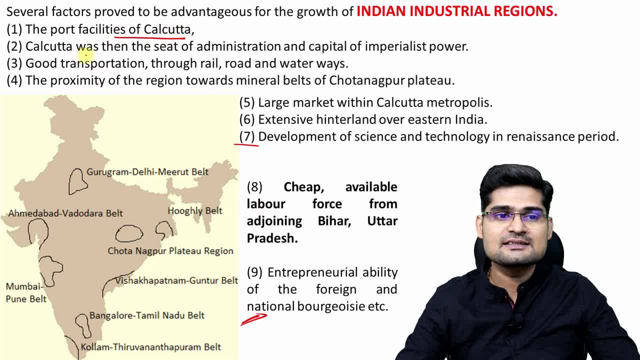 are available. that facilitates india. so port facilities right, for example kolkata port, right the earlier one. you have hugli belt here, then you have good transportation facility through rail, road, waterways, then you have mineral hub in chota nagpur region. you observe here this play to part. 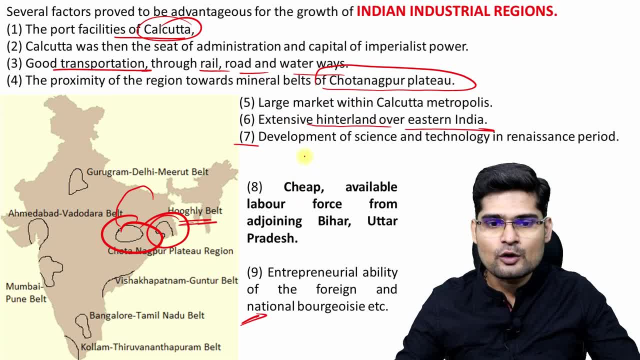 then you have extensive hinterland over eastern india and also science and technology development that led to this kind of hub development right, cheap available labor force, right. so all the labor is concentrated here in north india, up bihar and several other areas and entrepreneur ability of the foreign and national bourgeois. that is very important. so right from the pre-british 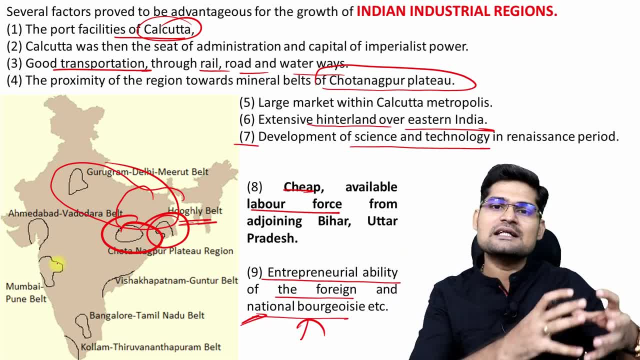 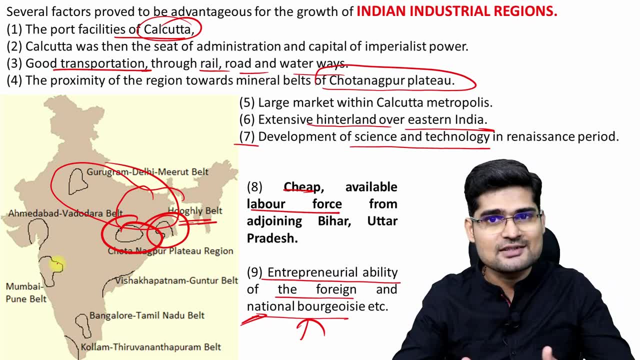 right from the moguls to british to current. you observe the industrial trend in india, right from the handicrafts and hand looms to the power looms to industrialization, now gradually picking up right. so that's what is happening and these are the major bells if you observe here clearly on 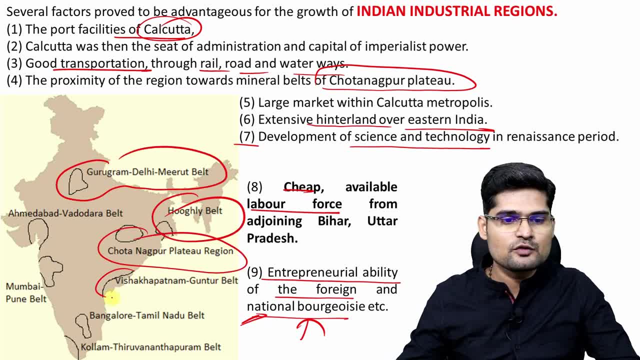 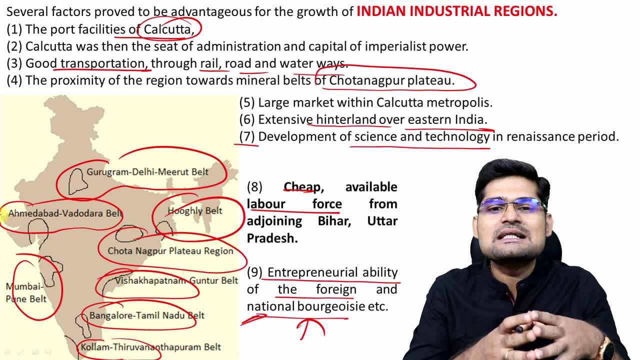 the map: gurugram, delhi, merit, hugli belt, chota, nagpur, play to vishagapatnam, bangalore, tamil nadu, column, tirunand puram, mumbai and amada buddhodra right. so these are the major bells in indian industrial. 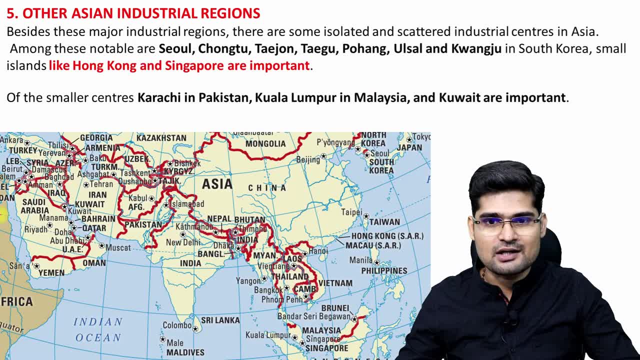 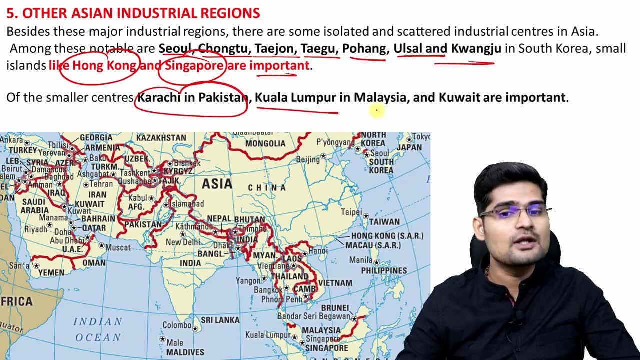 region for that matter. now comes to the other areas in asia. right, what are those? suol chongtu, tejon, tegu, pohang, ulsal and several others, and also hong kong and singapore, are the most important ones as well. apart from that, you have karachi in pakistan, kuala lumpur in malaysia and kuwait. these 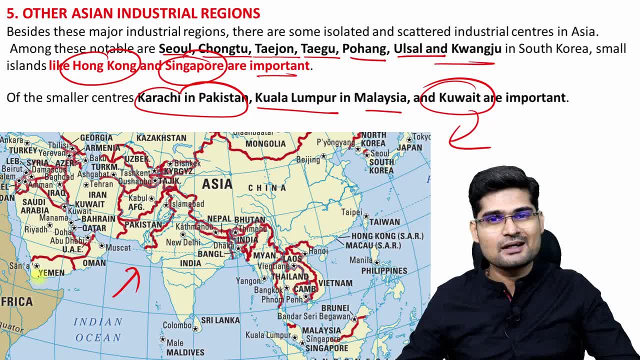 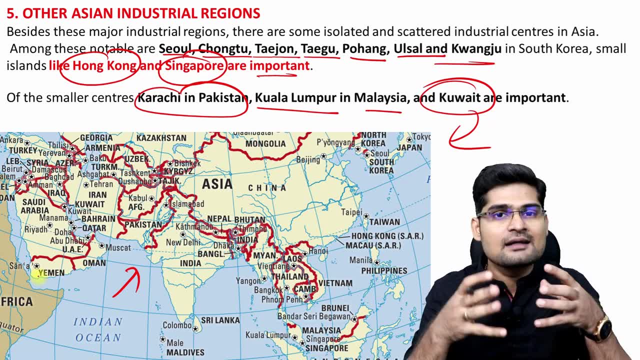 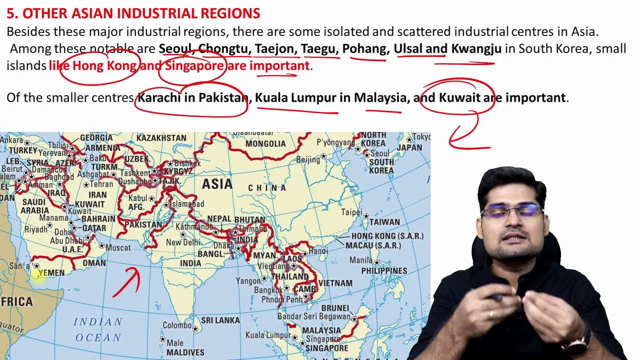 are the other centers. you can locate them on map right. these are the major hubs in asia. this is the distribution in other portions of the asia, apart from what we saw in china and in india. so what we learn here is the overview of the world manufacturing hub: how it is there, what are the 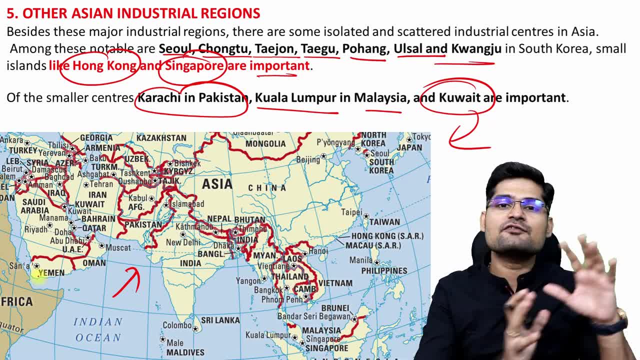 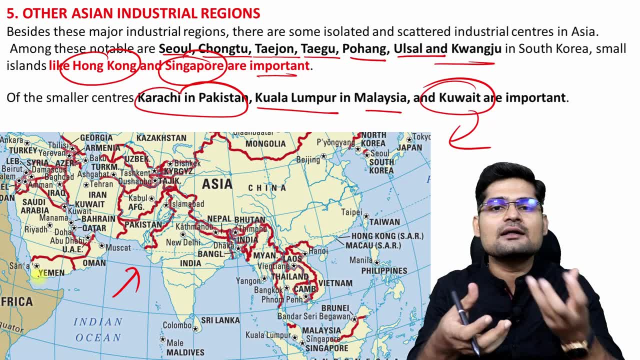 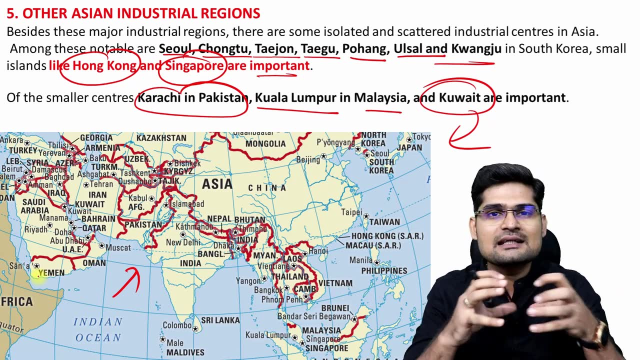 locational factors involved, where it is distributed, right from the north america, south america to europe, to asia, to the other portions in asia, right, so you can figure out a world pattern and also you can understand india as well, if you really want to make it to the answer writing so you can. 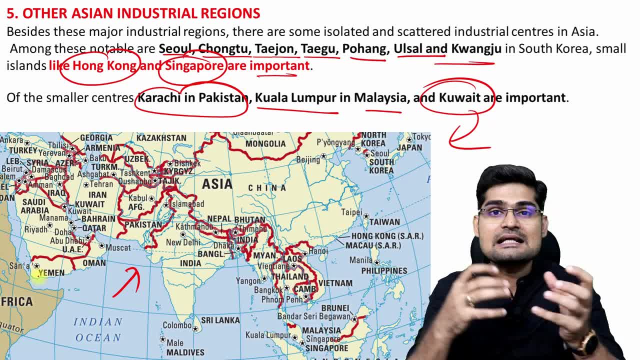 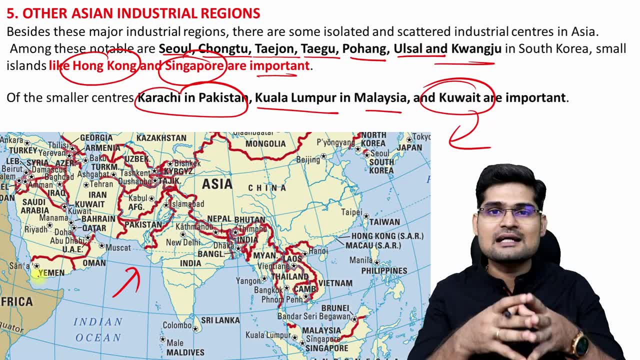 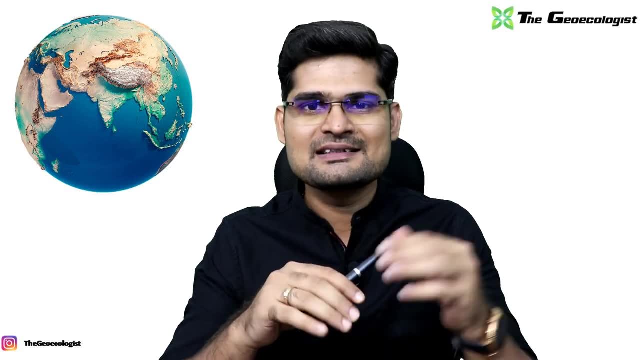 understand this entire picture of manufacturing units, their products they're leading in the market. in which sector are they leading? which kind of produces, specialized, where, that you can figure out and understand through maps. that's what the purpose of this lecture was. so now, when we have understood in details about the world manufacturing regions and also indian manufacturing regions, 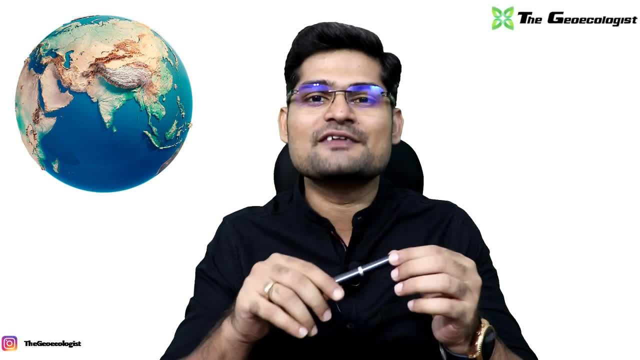 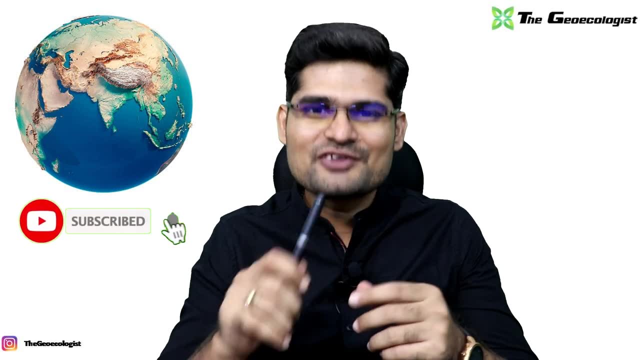 in the sessions to come, we'll be talking about various other topics of economic geography, special economic zones and others. so stay tuned, keep learning, keep watching and don't forget to subscribe to our channel and share the videos with others as well. 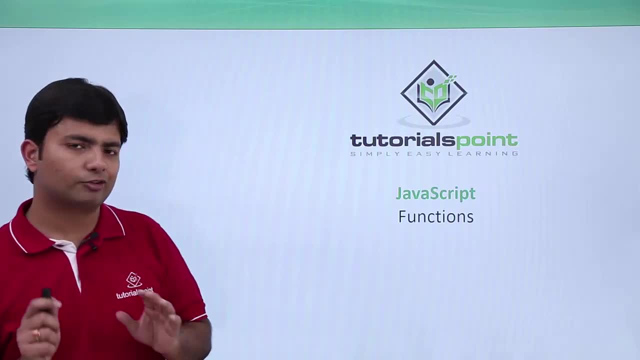 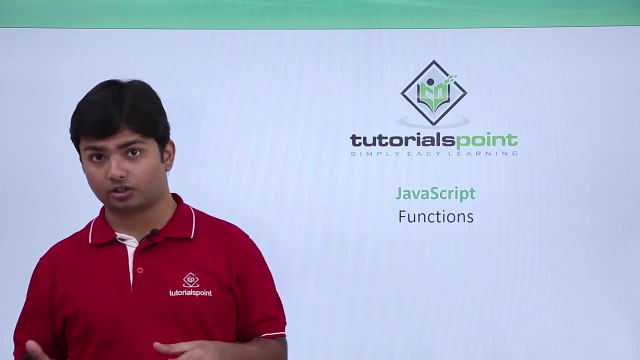 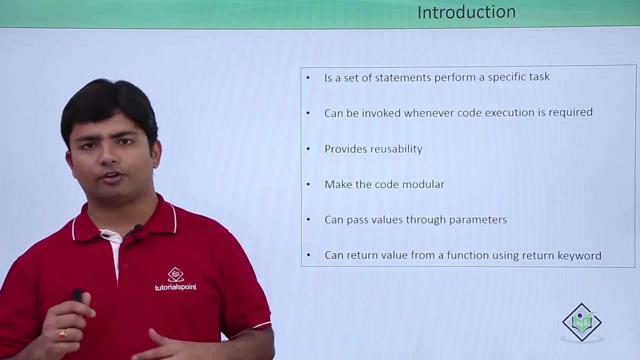 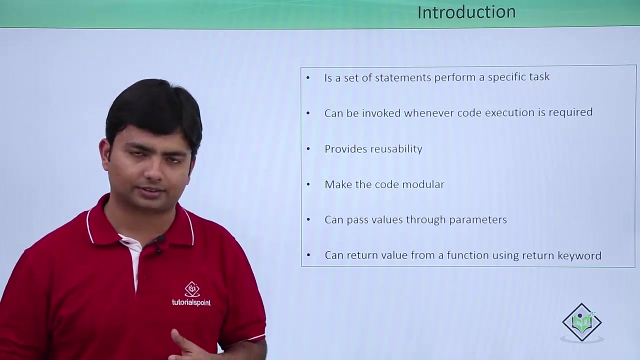 In this video of JavaScript, we are going to begin a very important concept called functions. As in the introduction, we have noticed that JavaScript is functional and now we are going to implement that thing. So what is a function? Basically, whenever I am talking about a function, it will contain a set of statements which perform a specific task.